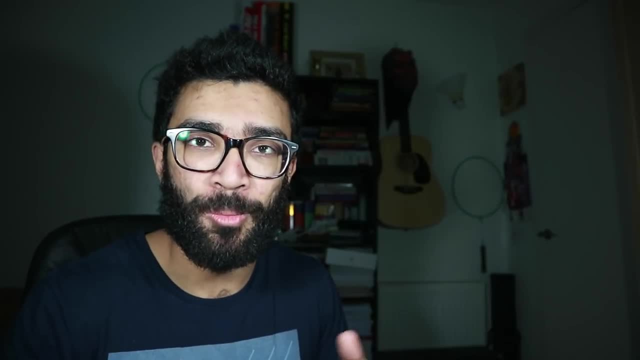 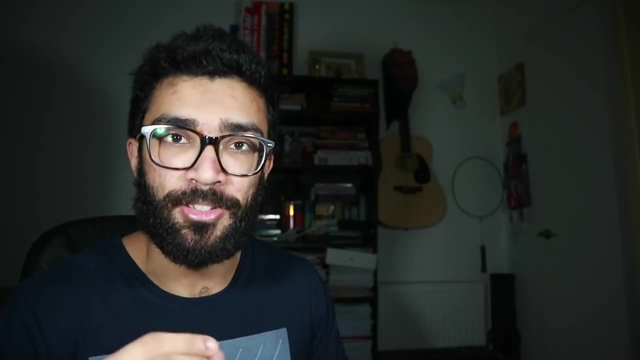 all, what even is it? Well, the uncertainty principle is a concept within the framework of quantum mechanics which, by the way, deals with very, very small objects. Now, the principle itself says something really baffling. It tells us that there is a fundamental and universal 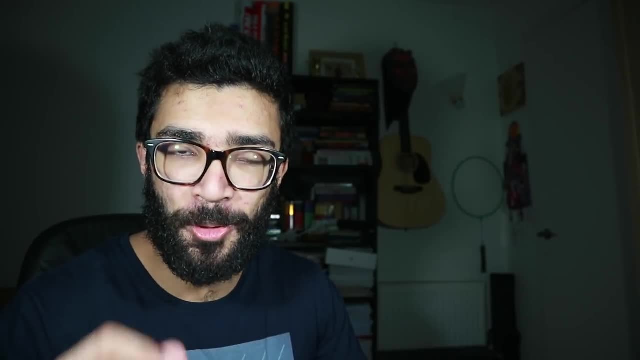 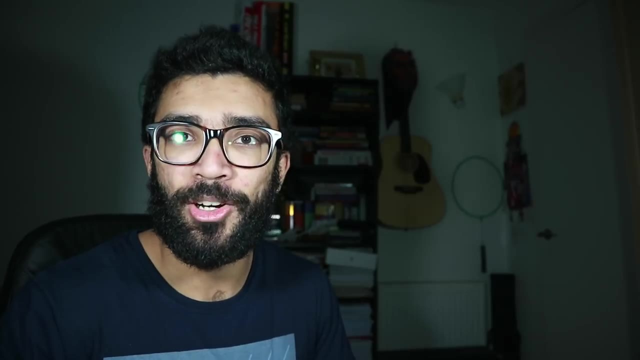 limit to how much we can know about pairs of quantities known as conjugate variables. Now, for our purposes in this video, conjugate basically means related to each other or linked together in a specific way, and variables are quantities that vary or change. Now, most commonly, the uncertainty 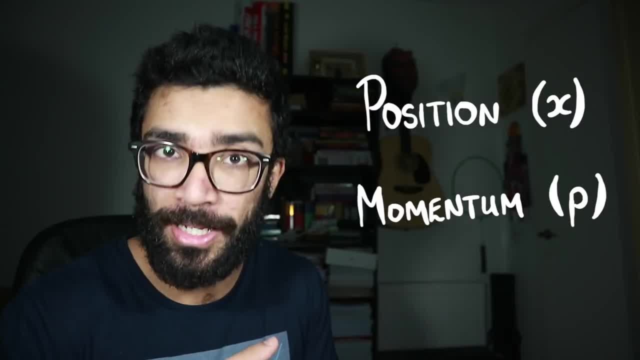 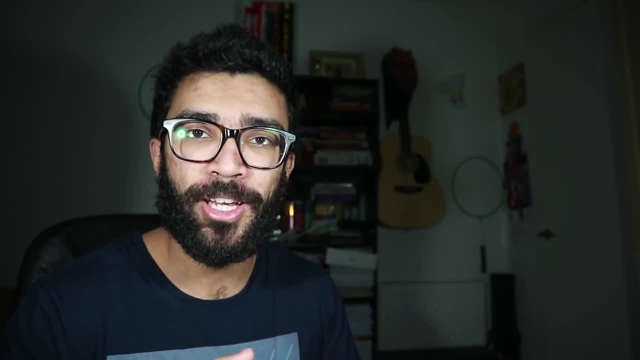 principle is described using the quantities of position and momentum. Momentum, by the way, is directly related to a particle speed. It's not exactly the same thing. there is a difference between speed and momentum, but for this video we'll kind of use the two terms interchangeably. 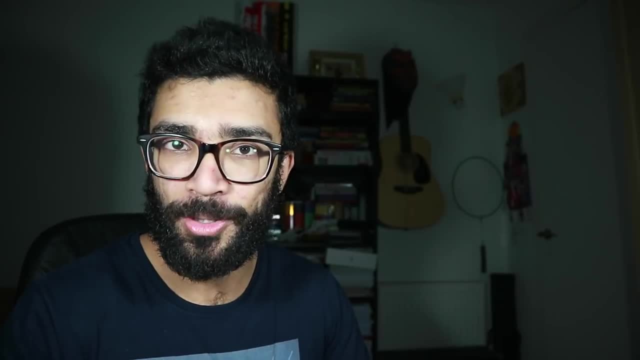 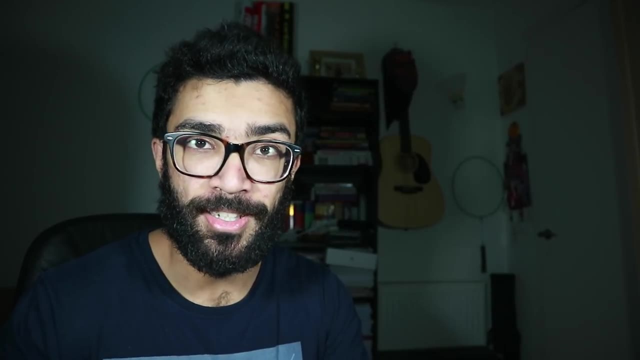 because they're very closely related, Related to each other. With these quantities, we're told that the more we know about one, the less we can know about the other. More specifically, then, the uncertainty principle tells us that if we take our uncertainty in position which we'll call delta x, 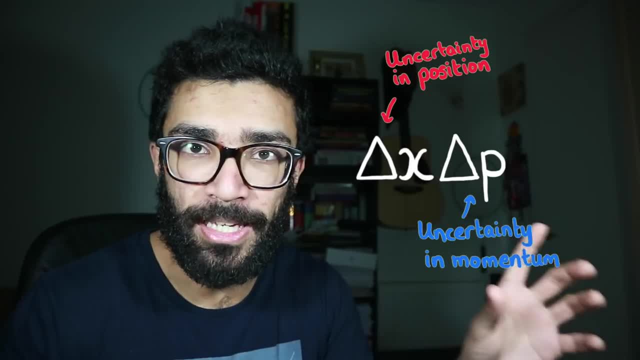 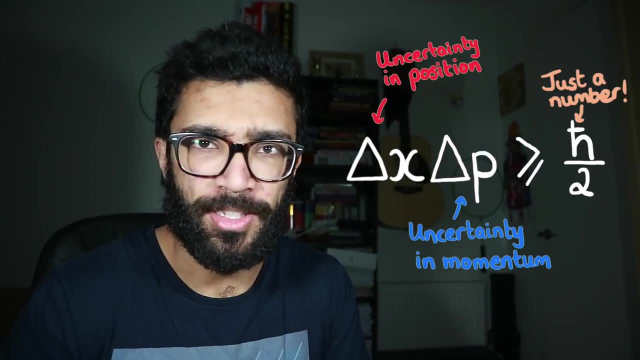 and multiply it by the uncertainty in momentum, which we'll call delta p, then this product, when we multiply these two together, is greater than or equal to h-bar divided by two. Now, h-bar is just a constant, it's just a number. So the right hand side of the inequality, h-bar. 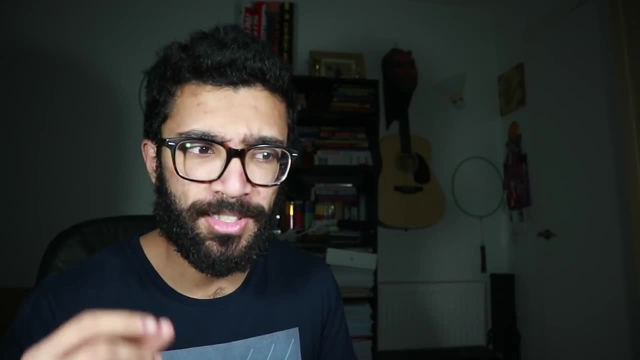 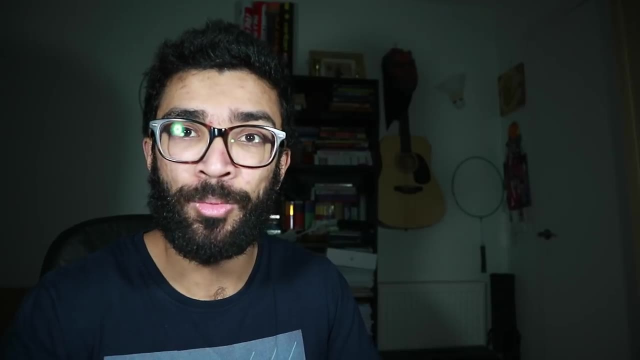 divided by two is also just a number. But let's think about this for a second. The uncertainty principle tells us that when we multiply the two uncertainties together, this has to be greater than or equal to some number. In other words, the product has to be at least this number. 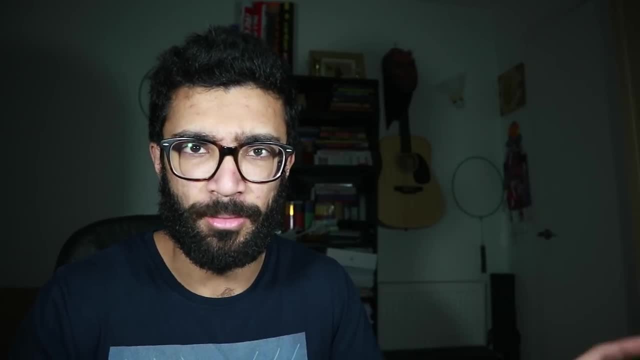 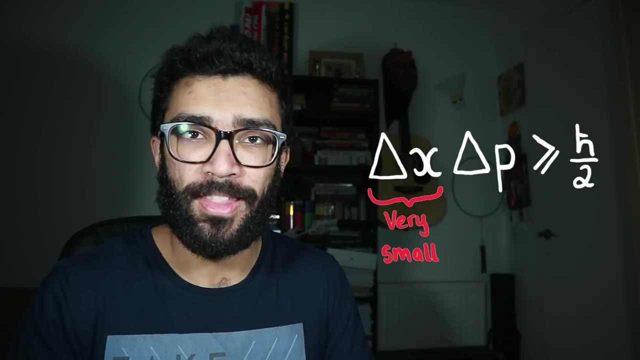 What does this mean, then? Well, it means that we cannot take the two quantities, delta x and delta p, and make them both as small as we would want them to be. If we make one of them small- let's say we make delta x very small- then the other quantity, delta p, has to get larger, so that when 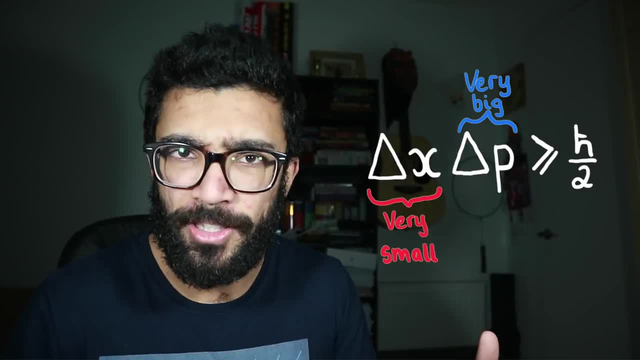 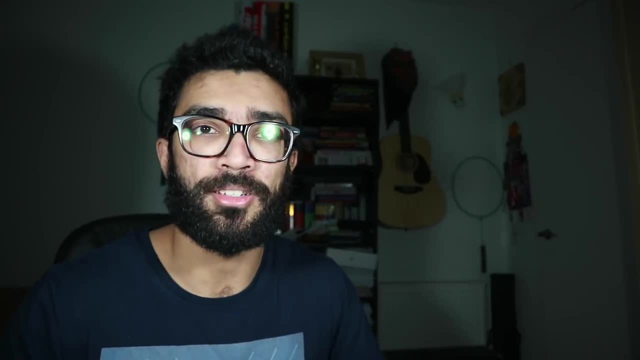 we multiply them together, it has to be at least h-bar divided by two. Why is this relevant to us then? Well, remember that these uncertainties represent uncertainties in our measurement of the position and the momentum of a particle, for example. Basically, here's a good way of thinking. 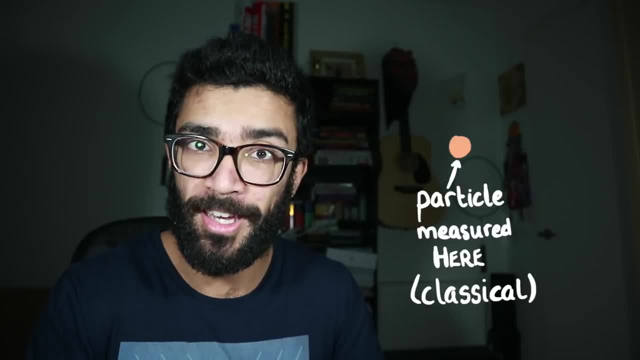 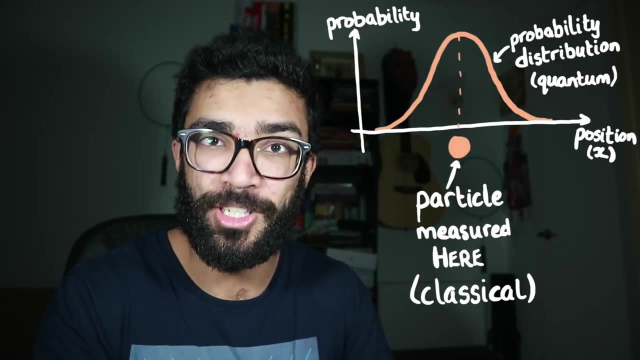 about it. Let's say normally in the classical world we would measure the particle to be here In the quantum world. it's not quite so simple. Before we measure the particle's position we have a probability distribution, usually peaked at the position that we would measure. 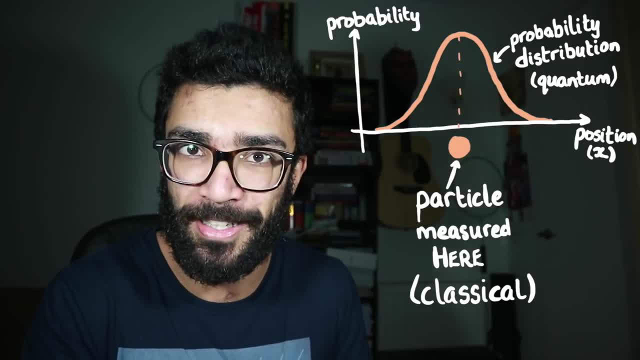 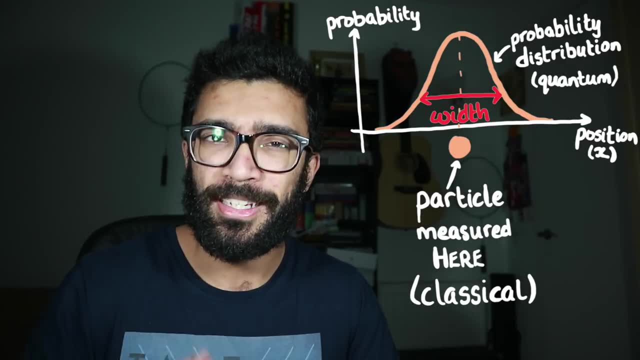 classically. In other words, there's a very high probability that the particle is where we would measure it to be classically. However, it also has a probability of being somewhere else, and it's the probability distribution, roughly speaking, that defines the uncertainty in our measurement of that. 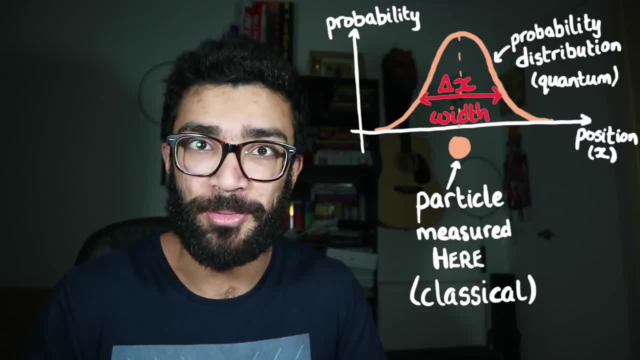 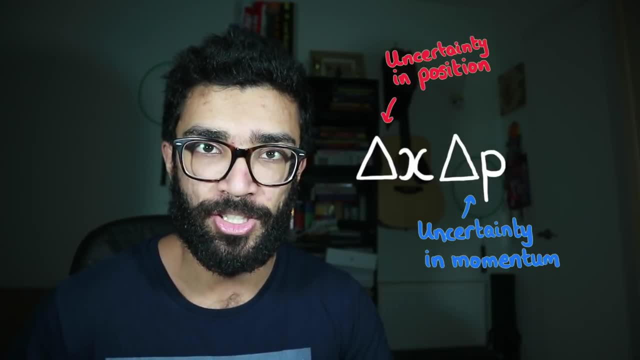 particle's position. In other words, the uncertainty is how uncertain we are about a measurement. So, coming back to our original point, then we cannot make both of these quantities delta x and delta p, the uncertainties in position and momentum. we cannot make them arbitrarily small. We can make 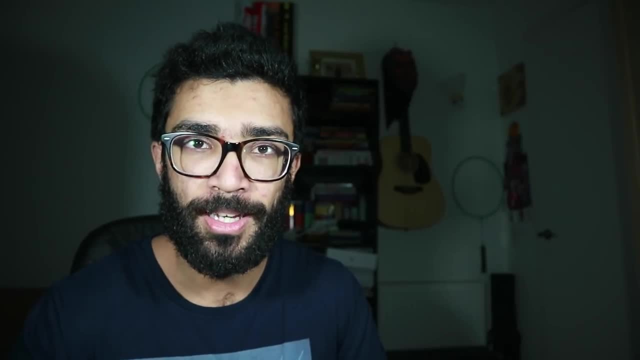 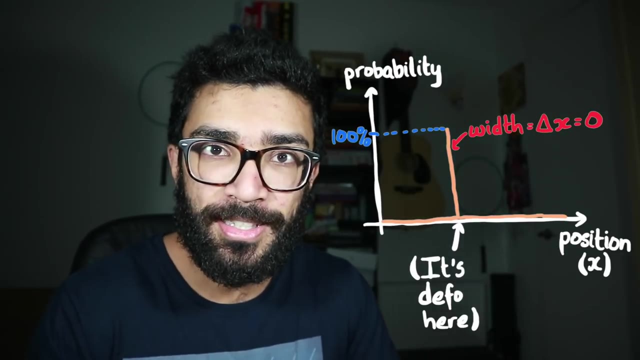 one of them arbitrarily small. We can't even make one of them zero. In other words, we know exactly where the particle's- let's say- position is, but that's at the expense of the other. If the uncertainty in the particle's position is zero, then the uncertainty in the particle's momentum- 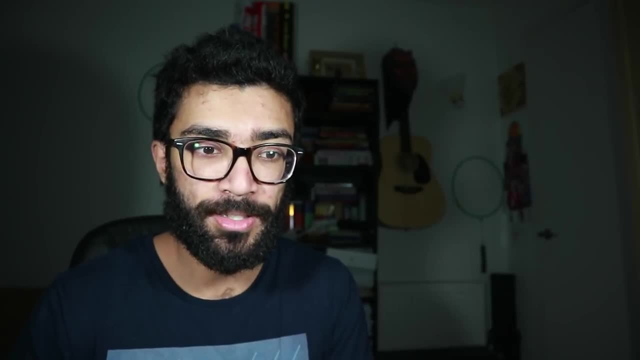 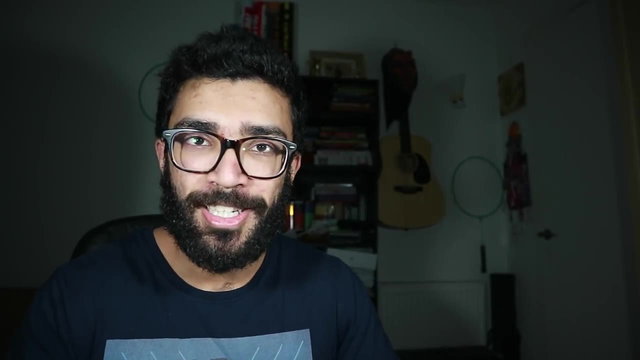 has to be infinity. In other words, if we know exactly where that particle is with 100 percent certainty, then we know absolutely nothing about that particle's momentum or speed. Now there's actually a lot I haven't mentioned about the uncertainty principle. I'm skimming over a lot. 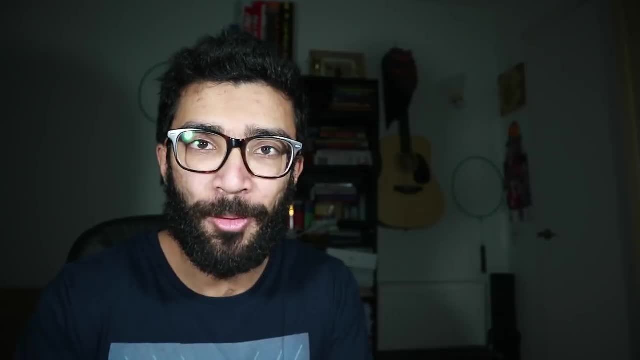 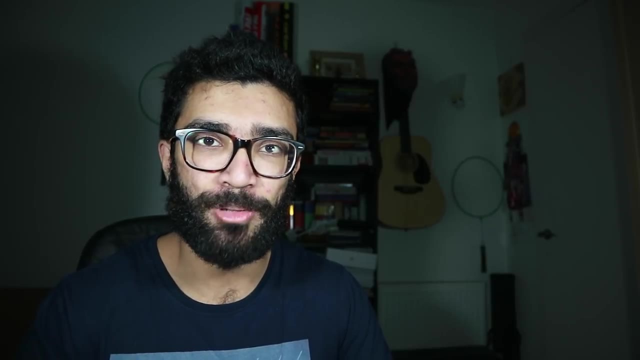 and simplifying a lot of things and taking away the subtlety out of a lot of things as well. I want us to look in some detail at where the uncertainty principle actually comes from. But before we go into that, let's look at a common description of the uncertainty principle that gets 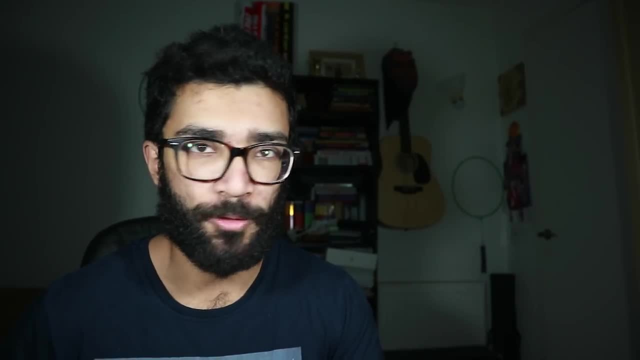 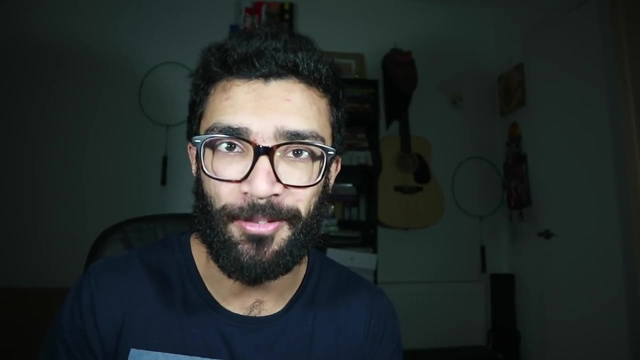 whenever the uncertainty principle is discussed. Okay, so let's consider we've got a particle. It's just doing its thing, sort of moving around in space. being a particle, How would we measure the position and speed of that particle? We can't just stick a ruler down beside it. It's teeny tiny. 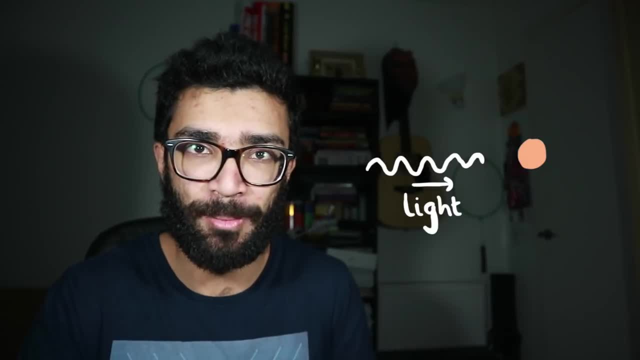 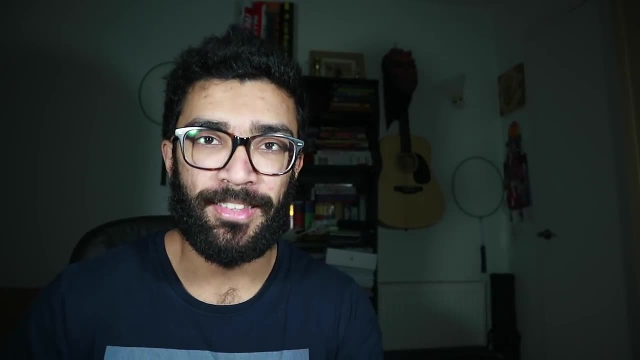 It's a particle. So what we have to do is to fire light at that particle. The light then bounces off that particle and gives us information about that particle's position and speed, or momentum. Now the interesting thing is, at this scale, at the teeny, tiny scale, quantum effects start to occur. 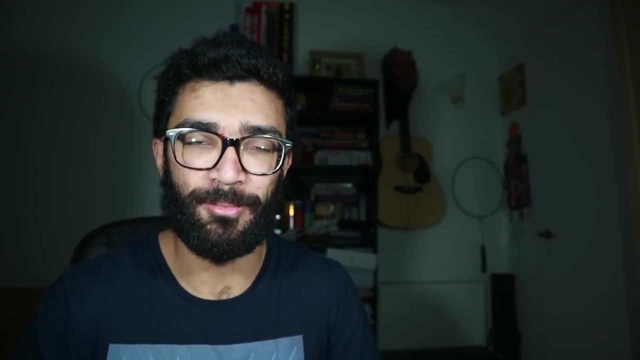 The light that we fire at it has quantum momentum. The light that we fire at it has quantum momentum properties. now, at this scale, It has wave-particle duality. Now, if you haven't heard of wave-particle duality, pause this video and google it, youtube it, wikipedia it. It's a really interesting and 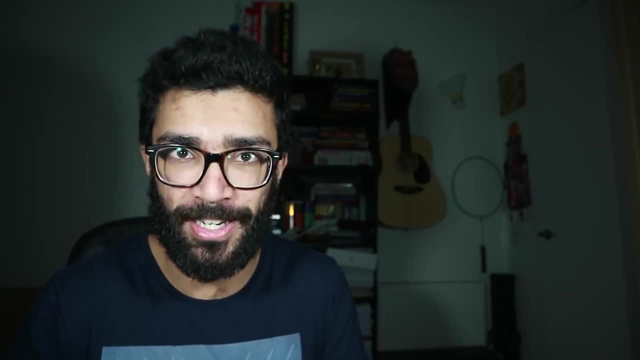 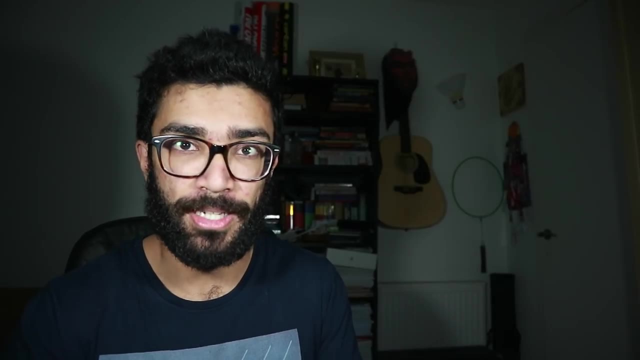 weird concept. There are a lot of good videos and explanations about it online, so go check it out and then come back to this video, But anyway. so wave-particle duality is the thing at those scales. In other words, when we fire light at this object, at this particle, the light itself will have both. 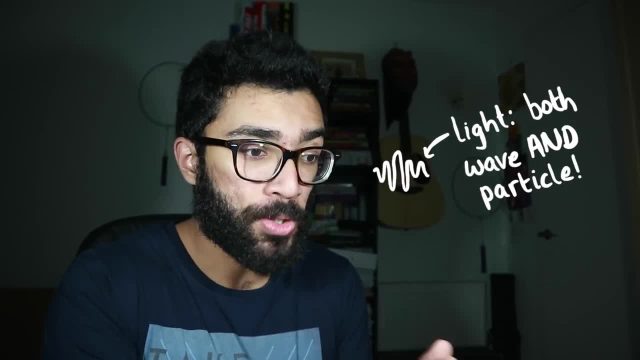 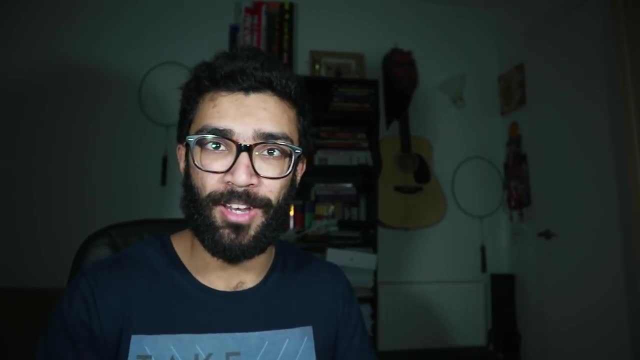 particle-like and wave-like properties. In other words, we'll be firing photons of light. Now, photons are particles, so we're firing particles of light at the particle that we're trying to measure. As well as this, because light has a wave-like behaviour, we can define that light. 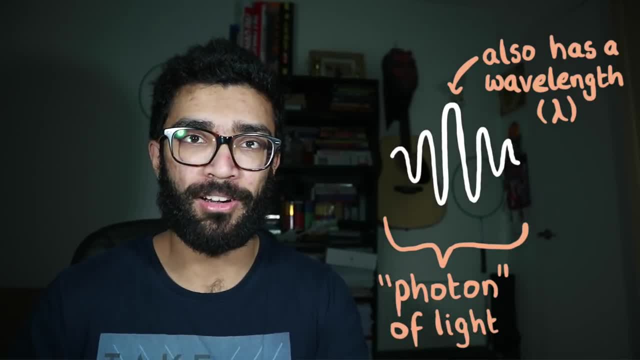 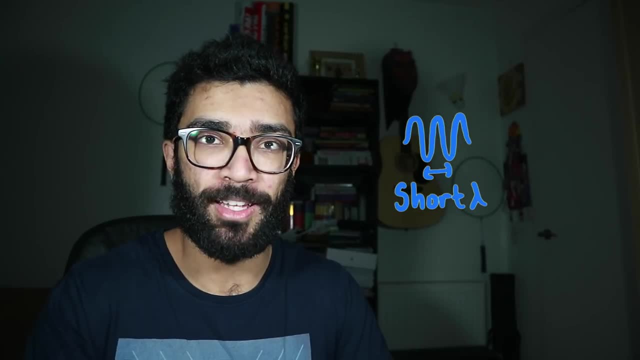 with a specific wavelength. Now, if the wavelength of the light that we're firing at the particle is short, if we have a short wavelength light, then we get more information about that particle's position, Because the peaks in short wavelength light are closer together. same thing with the. 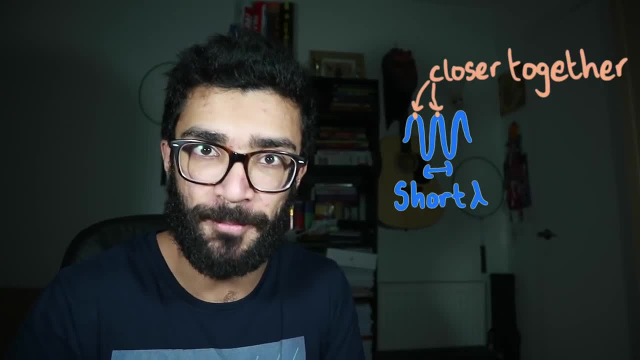 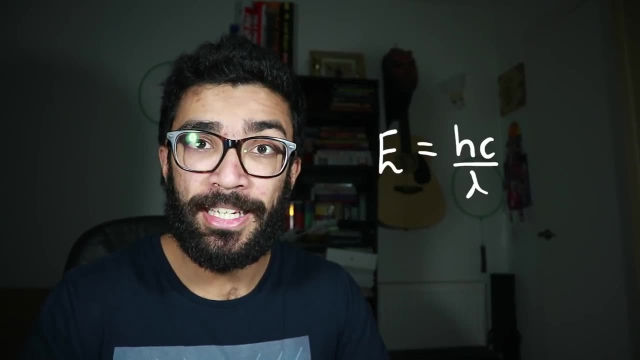 troughs, so we get more information about the whereabouts of that particle. However, this comes at a price. Remember that short wavelength particles are high energy particles. We can see this from the relationship: e is equal to hc divided by lambda. e is the amount of energy. 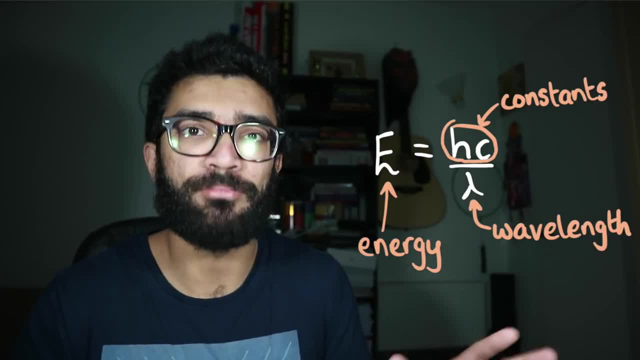 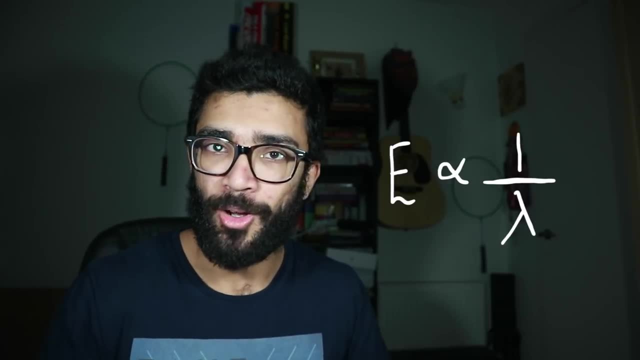 carried by the light. h and c are both just constants, just numbers, we don't need to worry about them too much. and lambda is the wavelength of the light. So in other words, e is inversely proportional to lambda. So if we have short wavelength light going into our particle, 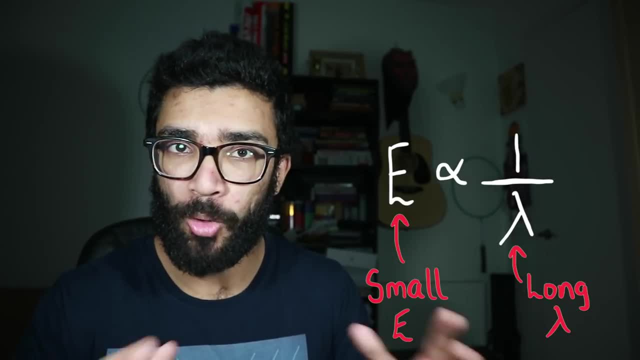 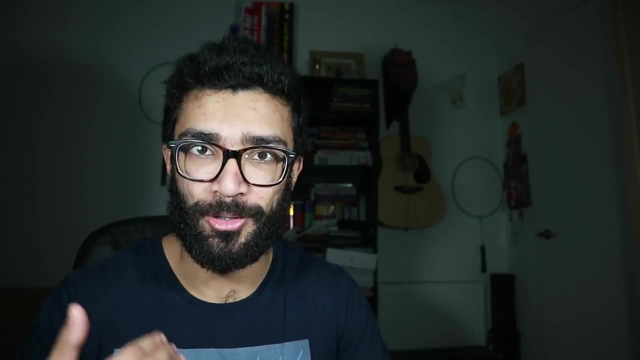 then the energy of that short wavelength light is large and vice versa, Long wavelength, small energy. So, as we said earlier, we're putting in short wavelength light into our particle. We get lots of information out about the particle's position. However, the light that we're 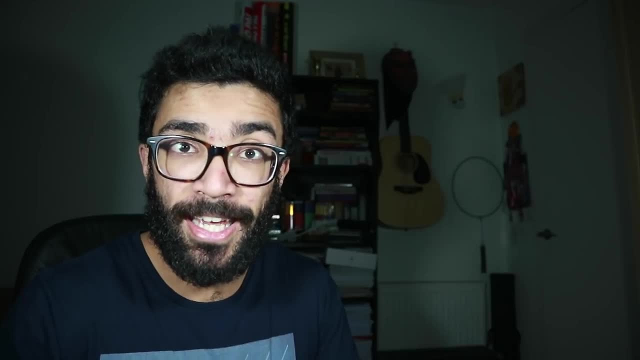 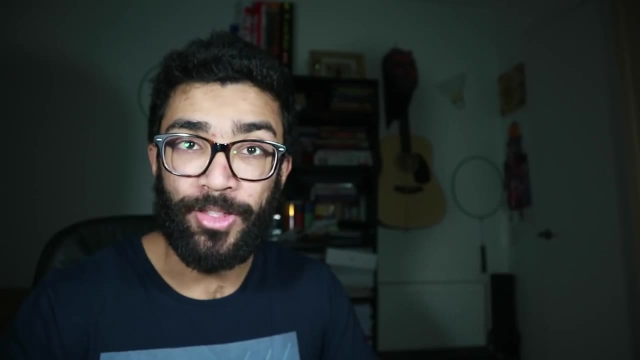 putting in short. wavelength light is high in energy, so it's going to result in a kick to the particle. The act of measuring it with that photon has resulted in a kick, and so we know less about that particle speed or momentum. Now this is the explanation that gets thrown around. 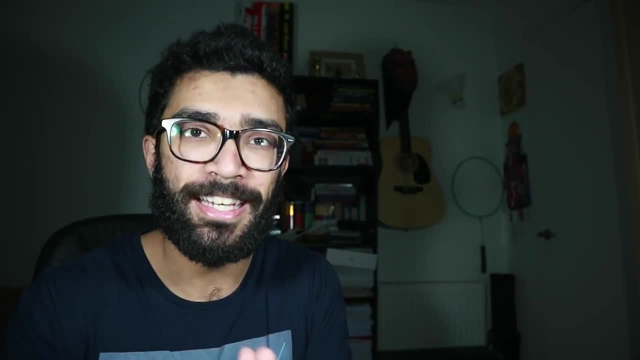 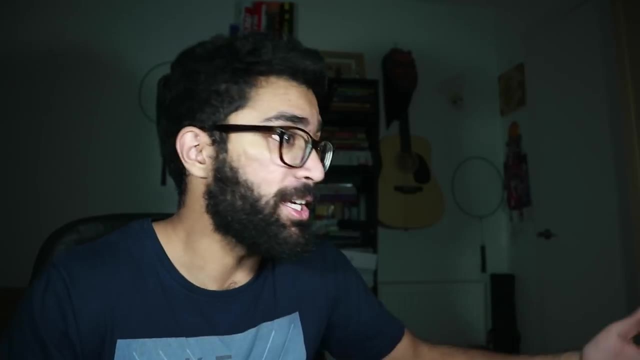 when Heisenberg's uncertainty principle is discussed. However, this is not Heisenberg's uncertainty principle. This is an explanation provided by Heisenberg as to why the uncertainty principle may be occurring. It's not an actual description of the uncertainty principle itself. 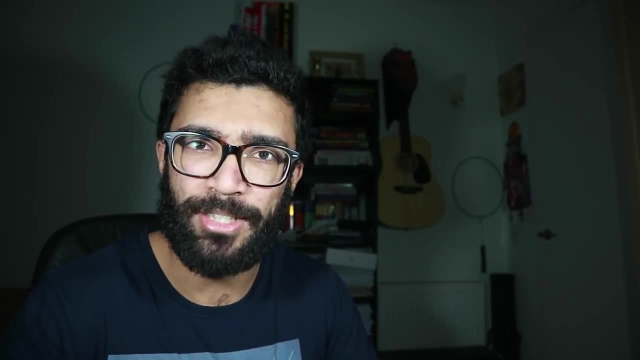 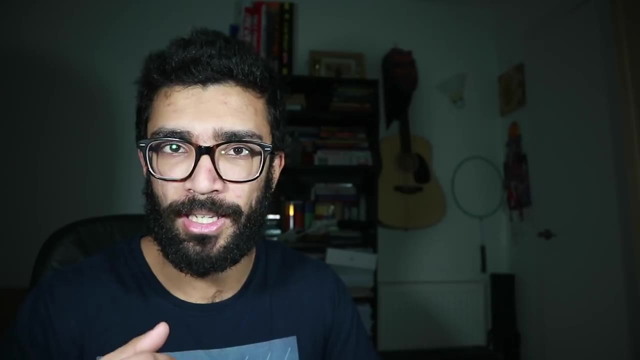 As well as this, it gets into a huge mess about how us measuring is making a difference to the particle's position or momentum, and blah, blah, blah, blah blah. Let's not get into that. And it also raises the question: well, why are we using light at all? Can't we think of? 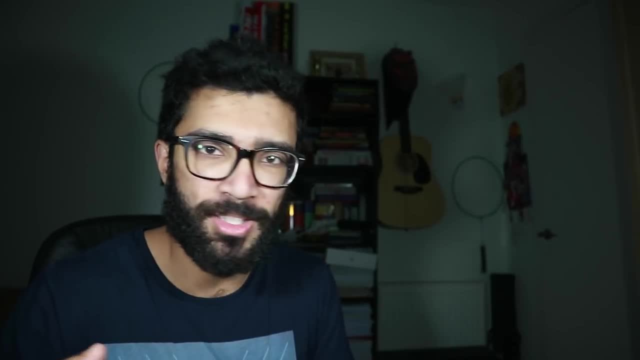 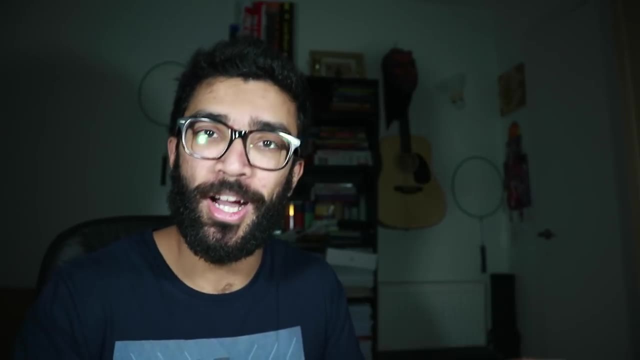 a better way to measure the particle's position and momentum. that would entirely subvert this problem. Well, that's the problem with this explanation. It's not the Heisenberg uncertainty principle, It's just a possible explanation as to why it occurs Instead. 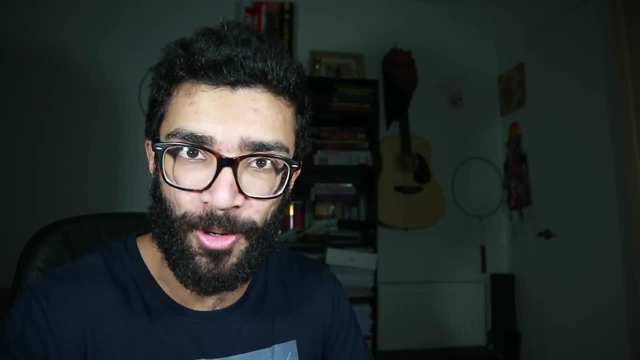 let's look at one of the ways of understanding where the principle actually comes from. Now, the way that I'm going to discuss of looking at the uncertainty principle will involve learning a little bit of maths. Specifically, we'll be looking at a topic 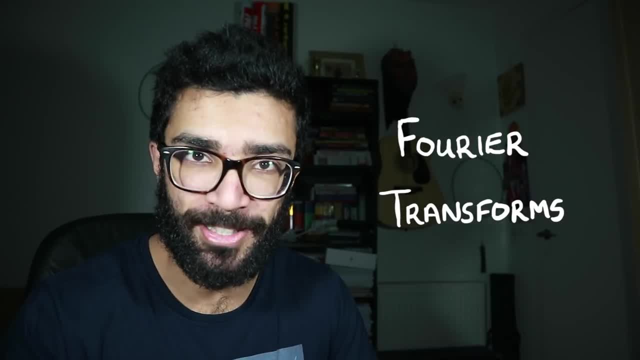 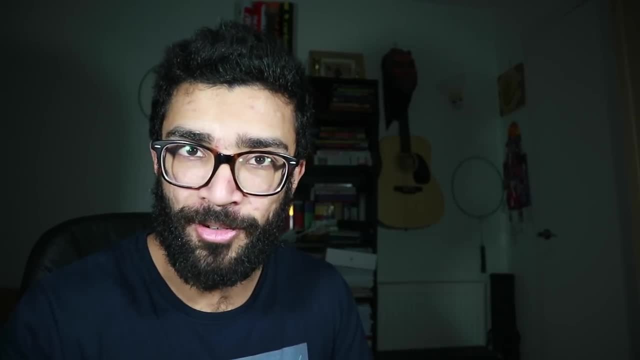 known as Fourier transforms. However, don't worry, I'll explain the basics of a Fourier transform using just pictures and English. We won't need to know any complicated maths or even go into any complicated maths. So Fourier transforms are based on a fairly simple concept. The idea is: 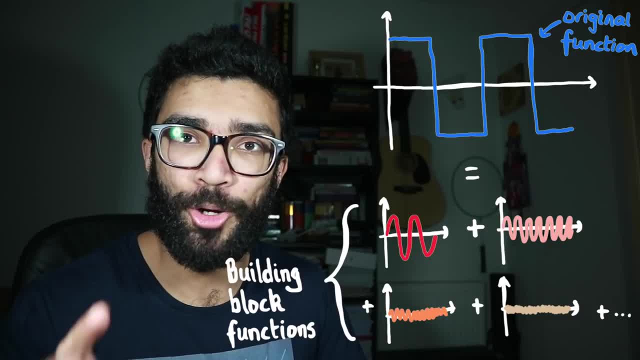 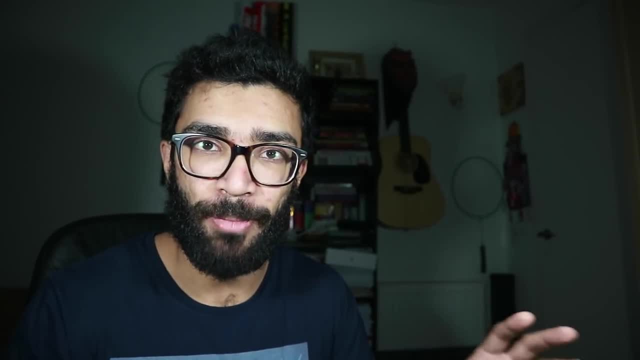 that lots of different functions, mathematical functions, can be broken down into building block functions, Confused. Let me give you an analogy to help. To find a good analogy, we need to look at another area of mathematics, specifically vectors. Now for those of you that have studied vectors, 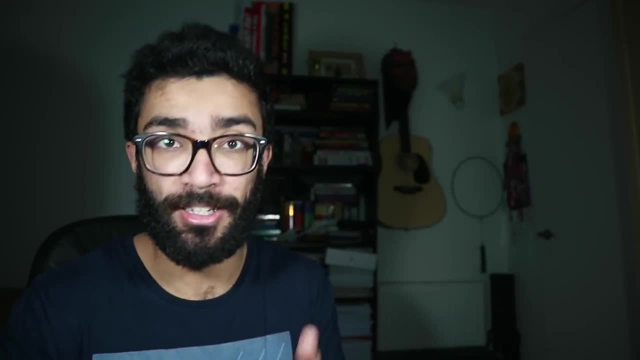 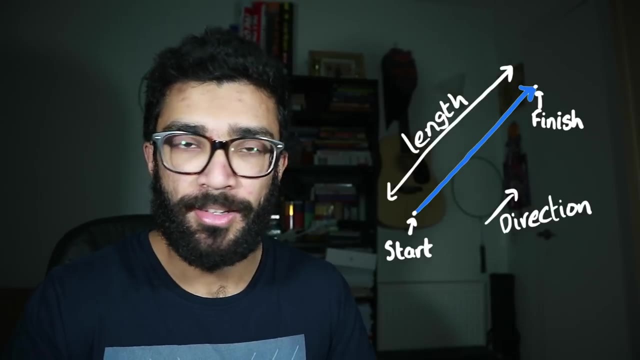 in any level of detail, you'll know that vectors have size and direction. So this arrow is of a representation of a vector. It starts at a certain point and it finishes at a certain point. It has a certain size- how long the vector is- and it has a certain direction, the direction in which 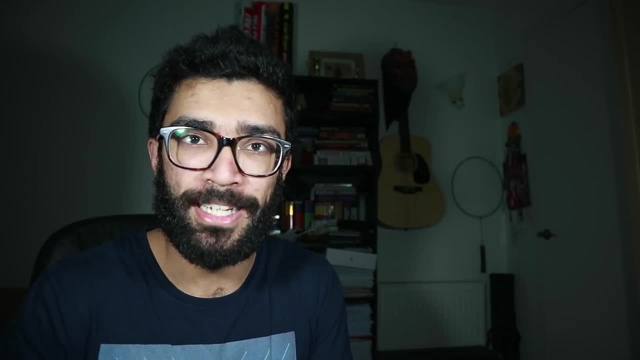 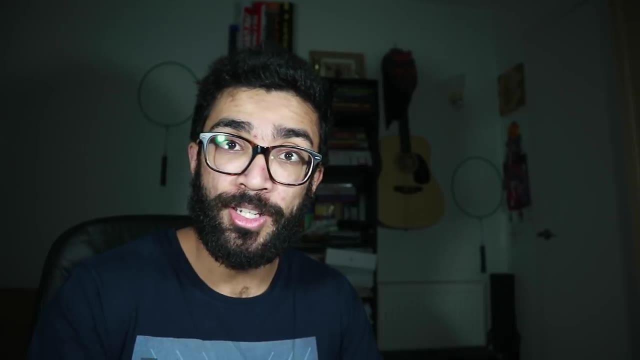 the arrow is pointing Now. many of you will know that we can take this vector and break it down into components. We can choose to break it up, for example, into its horizontal component and its vertical component. So let's say that our original vector was a size of five units long. 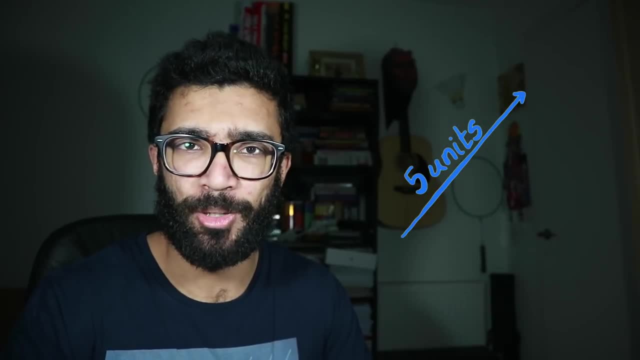 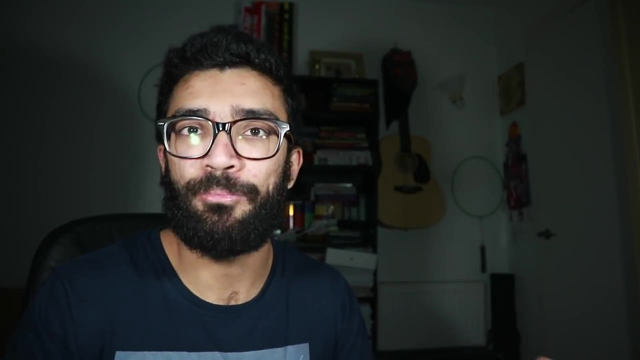 Now, how long one unit is doesn't matter. It could be a millimetre, it could be a centimetre, it could be a kilometre, it could even be a yard- for my American friends out there It doesn't matter. but let's say, our vector that we're looking at is five units long. 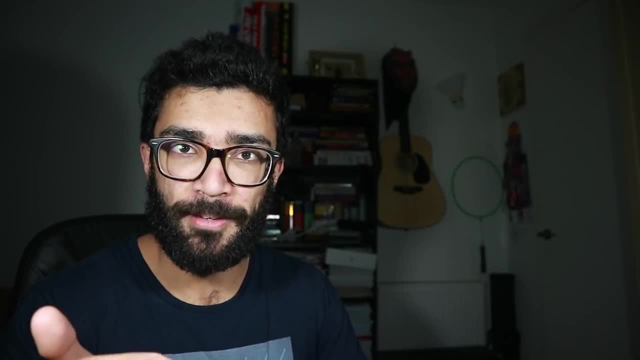 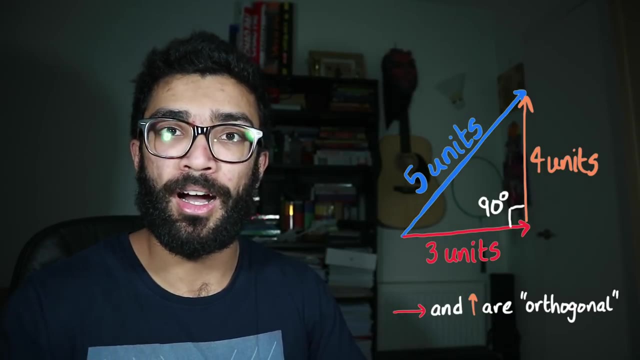 Now we can choose to break it up into its horizontal and vertical components. like I said, In this case the horizontal component is three units long and the vertical component is four units long. Now the horizontal and vertical components are at 90 degrees to each other. The 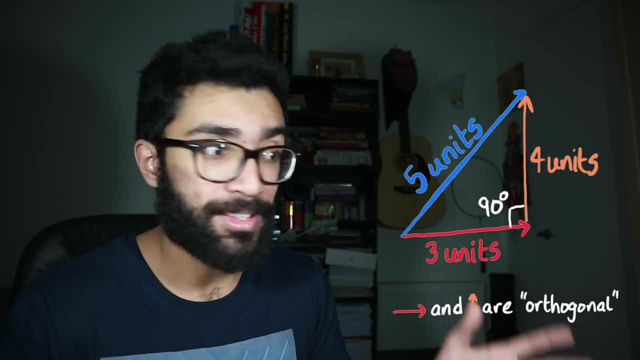 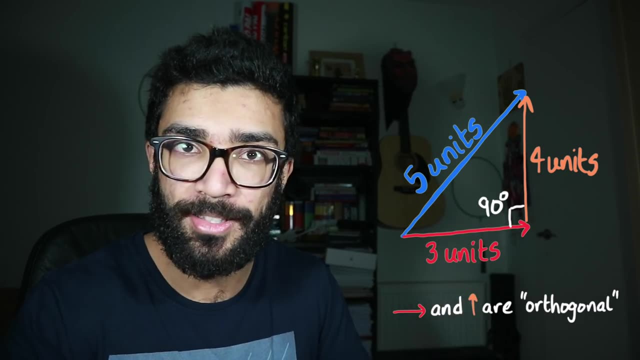 technical word for this is they're orthogonal to each other, which means that the triangle that we've just drawn is a right-angled triangle, And hence we can apply Pythagoras's theorem to ensure that the lengths of the sides of the horizontal component, the vertical component and the original 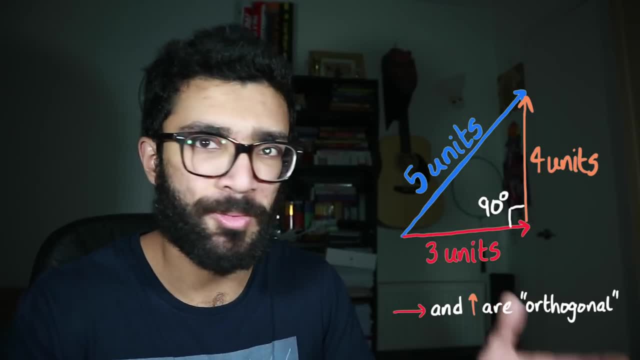 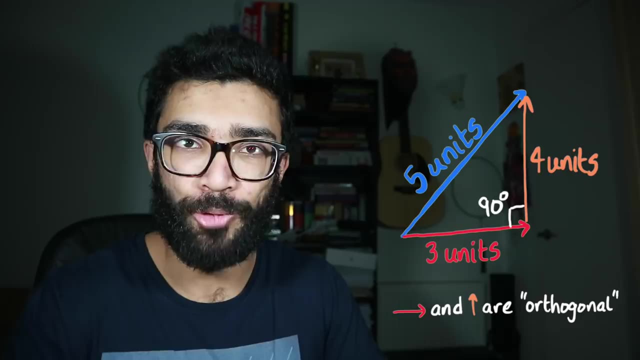 vector do actually work out. Try it for yourself. Apply Pythagoras's theorem to the side lengths of this triangle, Anyway. so basically, what we've done is we've taken this vector, the original vector that's five units long, and broken it down into a horizontal component which is three units long. 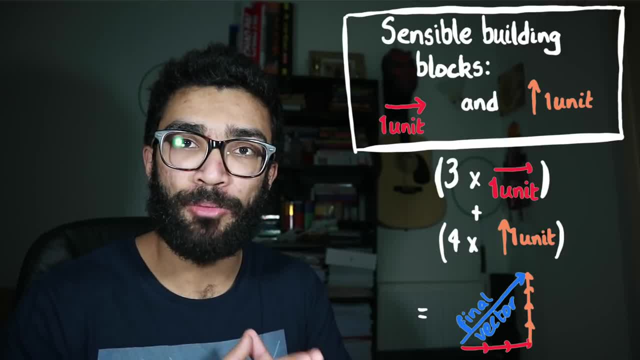 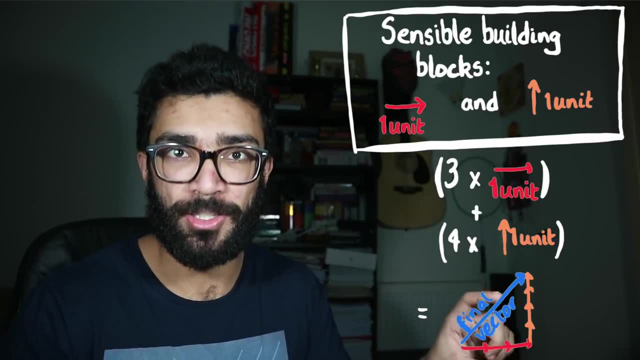 and a vertical component which is four units long. So, basically, we've taken our vector and broken it down into sensible building blocks, the sensible building blocks being a unit-long vector in the horizontal direction and a unit-long vector in the vertical direction. We've got three in the 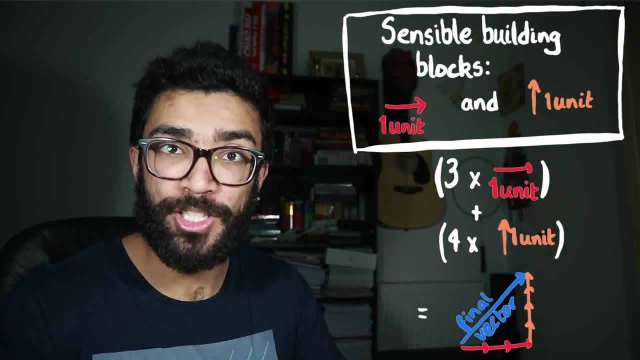 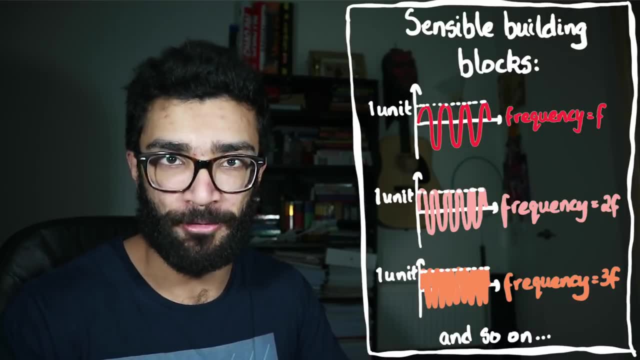 horizontal and four in the vertical. Just like that, we can break a function up into sensible building blocks made up of different functions. Specifically, the functions that we'll be using as building blocks will be sine waves of different frequencies. They're also unit sine waves by the 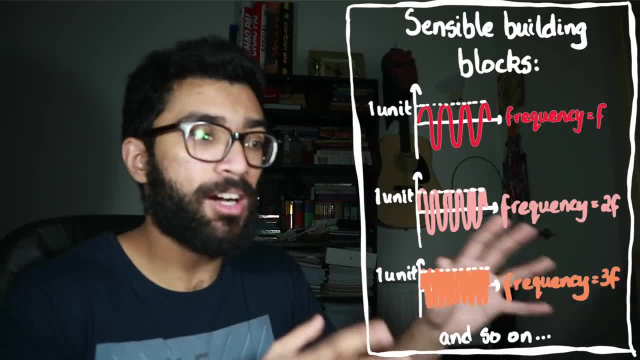 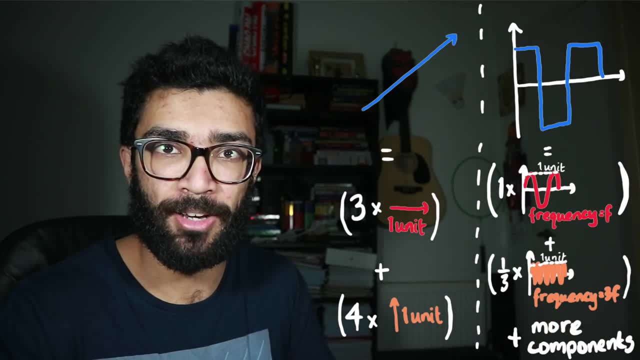 way because their amplitudes are one. And basically, what we can do is to take our function and break it down into different amounts of sine waves at different frequencies, just like how we took our vector and broke it down into different amounts of horizontal vector and vertical vector. 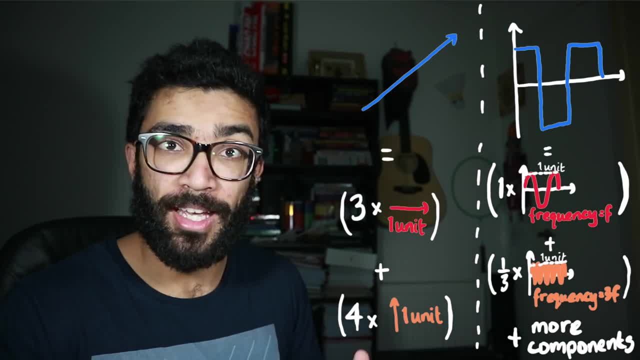 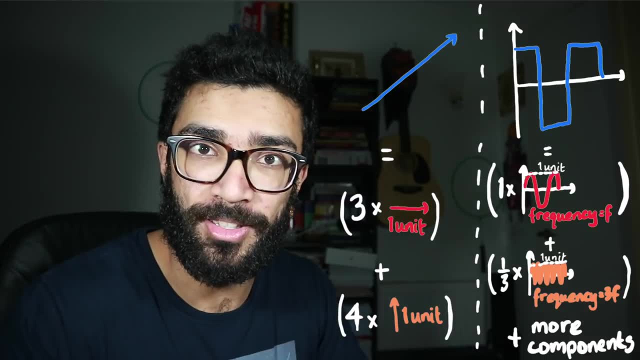 In this analogy, our original vector is our original function. The sine wave at one frequency is one of our sensible unit vectors. The sine wave at another frequency is another one of our sensible unit vectors, and so on and so forth. If we want five units of this, 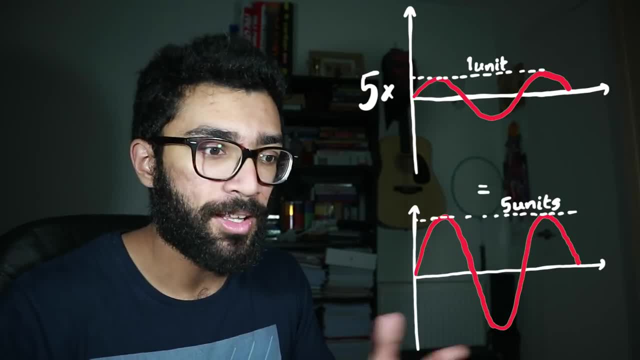 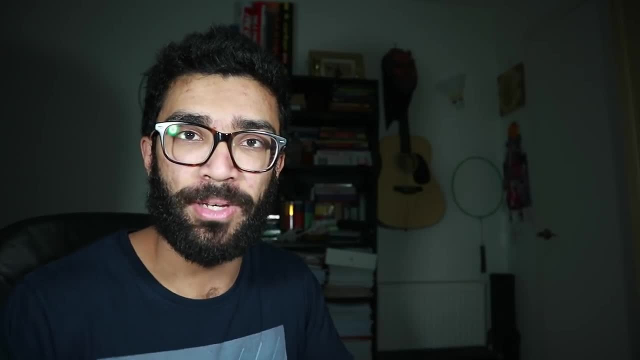 sine wave, we just multiply its amplitude by five, Then we add it to another sine wave with a different frequency. That's the analogy. By the way, interestingly, the sine waves of different frequencies are defined as being orthogonal to each other, just like how we had the horizontal. 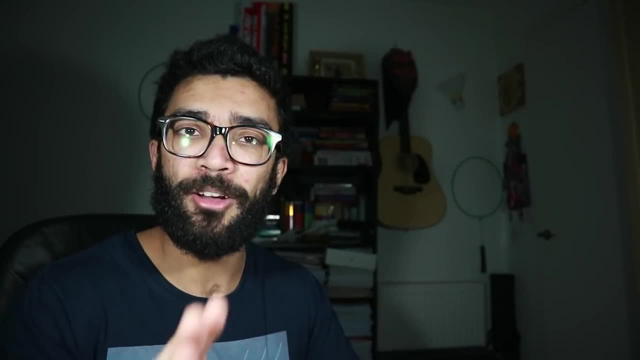 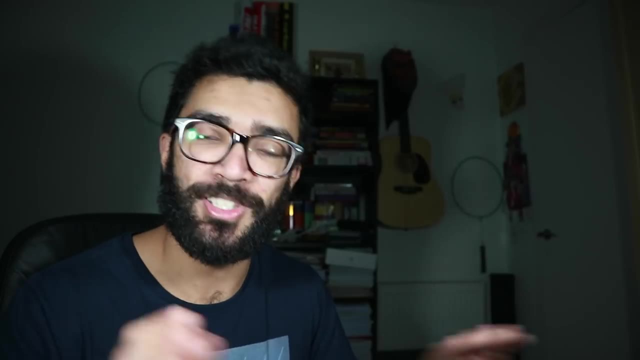 unit vectors and the vertical unit vectors being orthogonal to each other. However, the definition of orthogonal in this case is different. They're not at 90 degrees to each other, but there's a really clever definition which I won't go into. Just take my word for it that they're orthogonal. 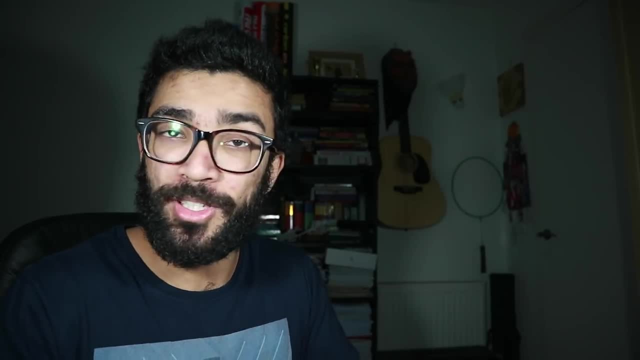 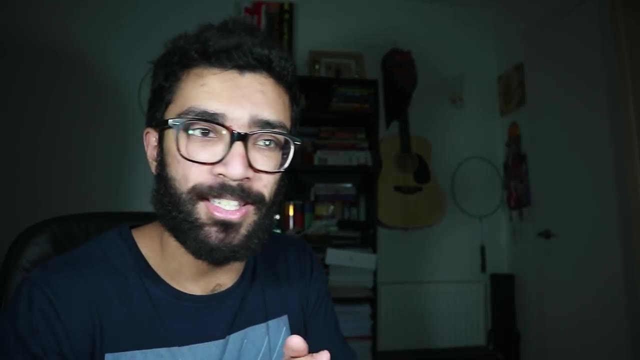 Also, if you don't know exactly what I mean by sine waves at different frequencies, pause this video and check out on the internet an explanation for the frequencies of waves. However, let's carry on. So we've taken our original function and we've broken it down into building block functions. Now 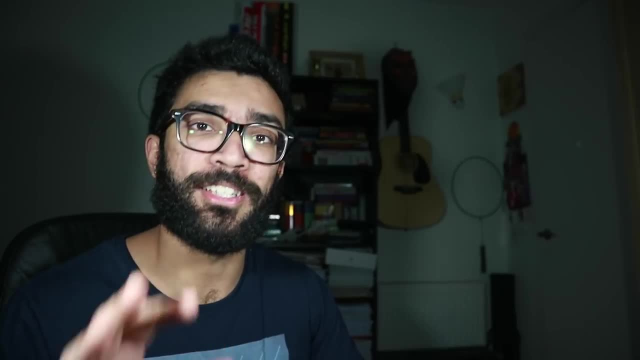 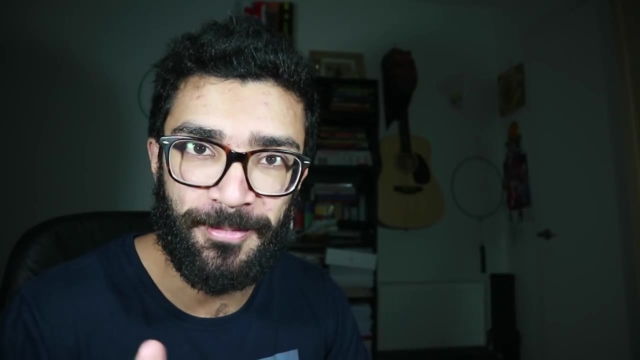 this is a really tricky concept, so feel free to replay this part of the video until you understand exactly what I'm talking about. If it's still not clear, please, please, please, feel free to drop me a comment below and I'll try and clarify as much as I can in the comments. Otherwise, feel free to. 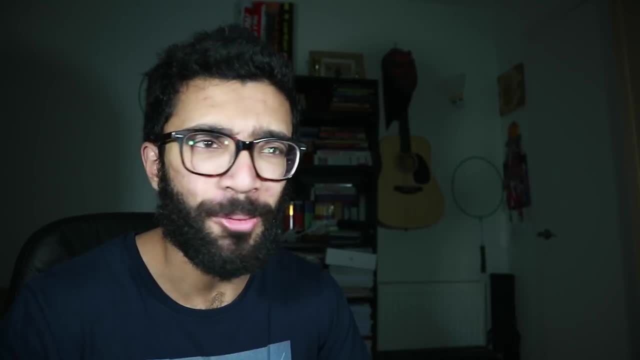 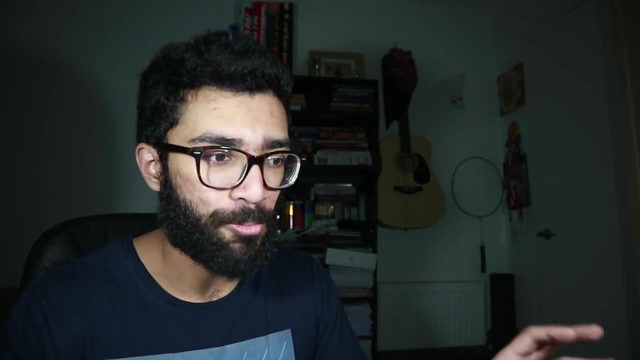 check out Fourier transforms on the internet, though I should warn you they're quite complicated Anyway. so the thing that's of interest to us when we break down a function into its constituent sine waves is that the sine waves that we break them down into are at. 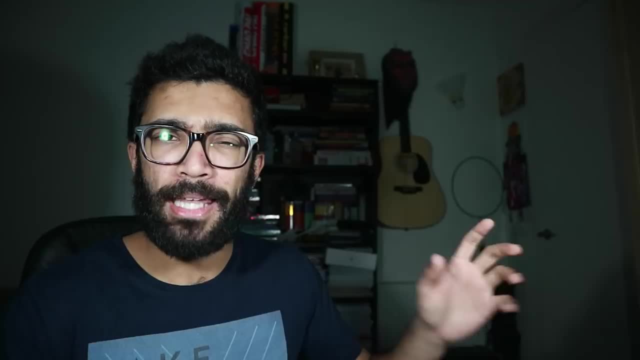 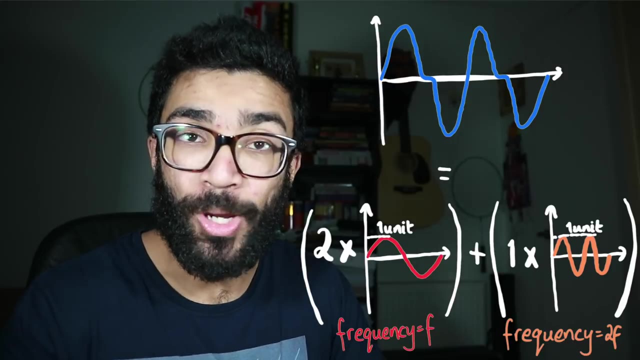 different frequencies. The reason for this is that we can do something really clever. Let's say we have a function which we can break down into two units of one frequency and one unit of another frequency, and nothing else. What we can do is to make a new plot, a new function On the x. 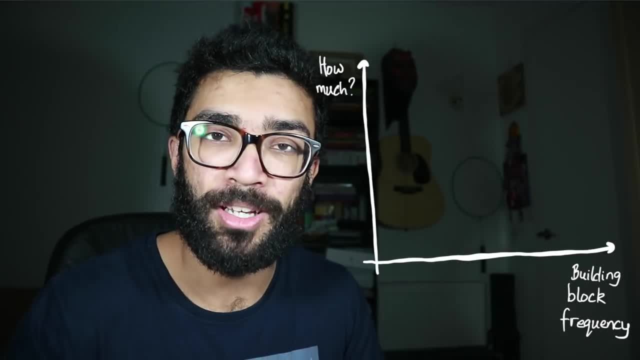 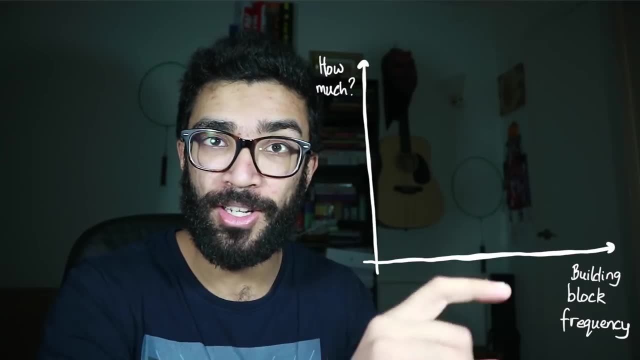 or the horizontal axis will be the frequencies of the components that we've broken our function into, And on the vertical axis will be how much of each component we have. So, like we said, in our function we had two units of the first frequency. 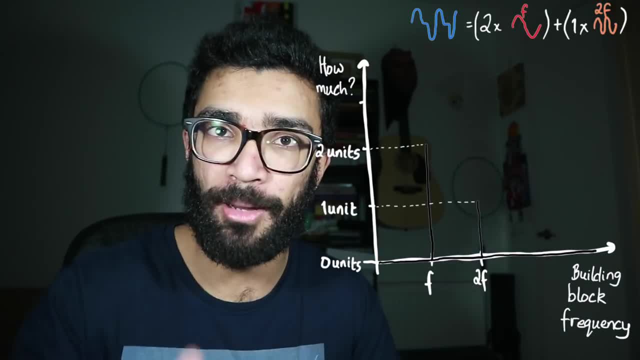 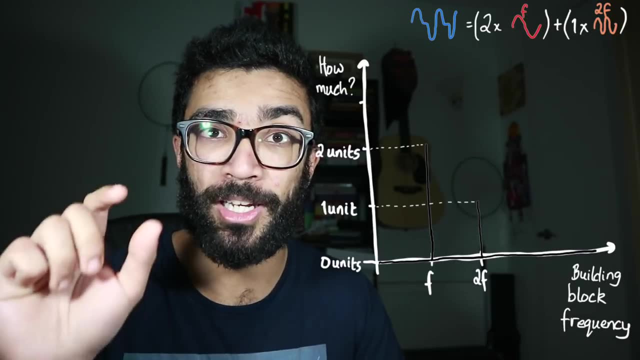 so we'll plot at the first frequency along the horizontal axis, two units up, and we have one unit of the second frequency. Now we have no other frequency sine waves in our original function. so for every other frequency on our new plot the amount will be zero. Now, at this point, what we've 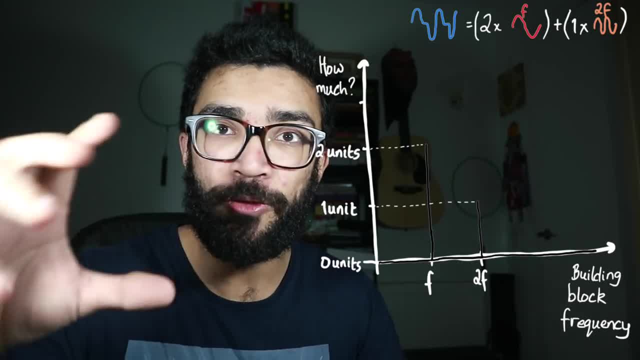 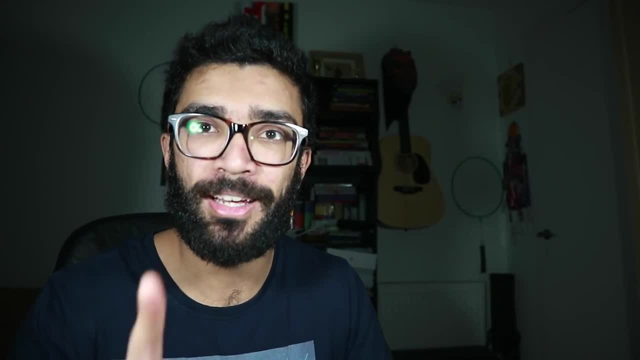 done is we've made a new plot, we've made a new function. This new function is known as a Fourier transform of our original function. We'll link it to the Heisenberg uncertainty principle in a second, but before we do that, there's an interesting thing to note about Fourier transforms. If 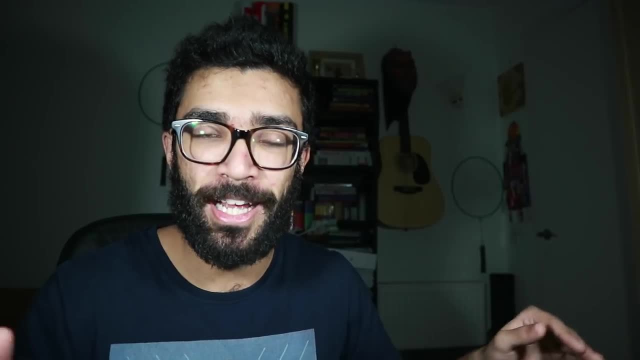 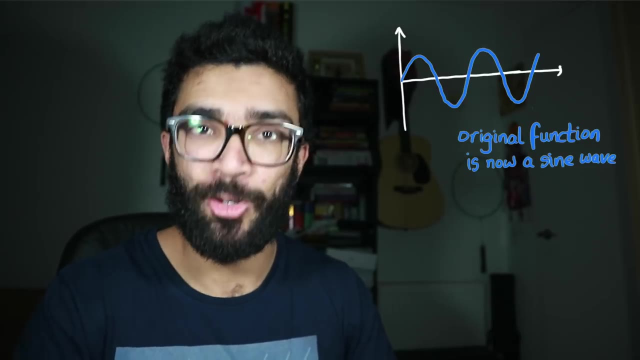 our original function is really really wide on its horizontal axis, then we're going to have a Fourier transform of that function that's going to be really really narrow. This is a property of Fourier transforms. For example, let's just take a normal sine wave. It's a pure sine wave, so it. 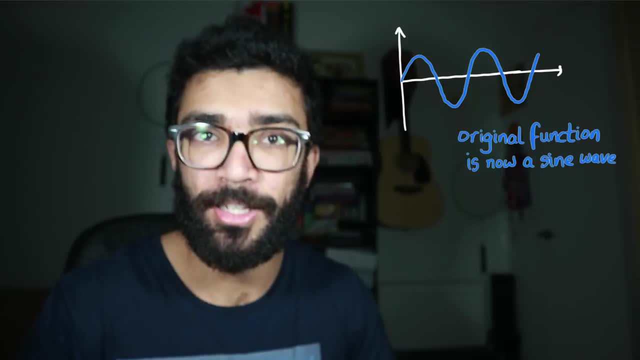 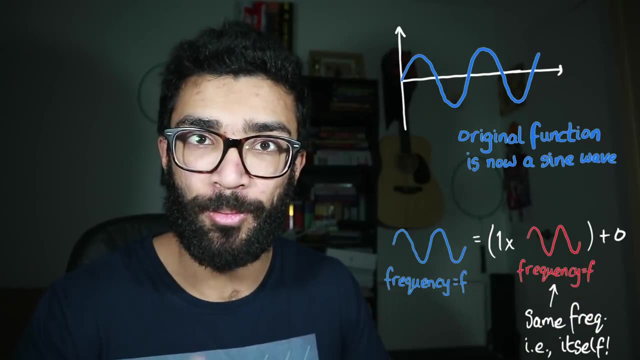 only has one frequency. So when we break it down into its constituent components, well, its constituent component is just itself. We've got one frequency, one sine wave, one pure sine wave. Now, a sine wave stretches on forever in the horizontal direction because it's a pure sine. 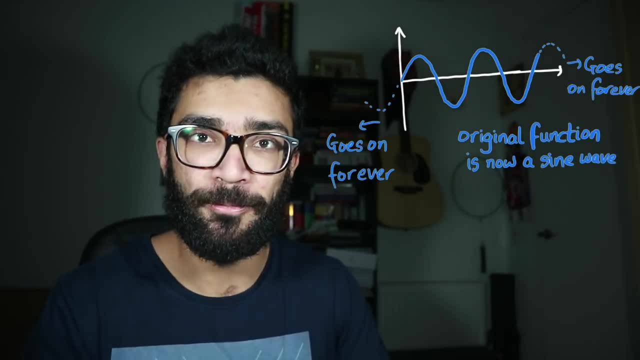 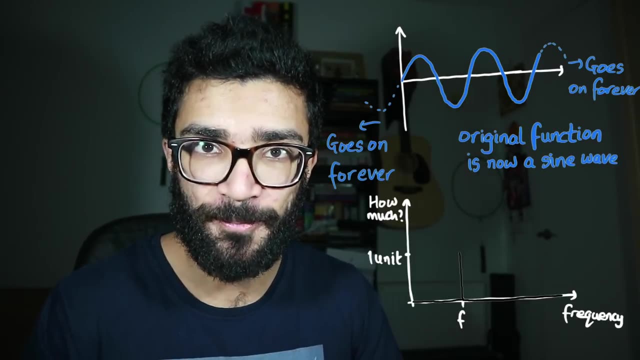 wave. It goes on forever in this direction and in this direction. Now, if we were to plot its Fourier transform, it looks something like this. So if we were to plot this Fourier transform, it looks like this because its components, its building blocks, are just made up of one frequency sine. 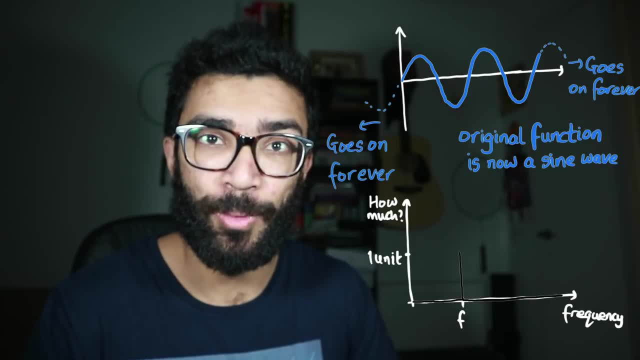 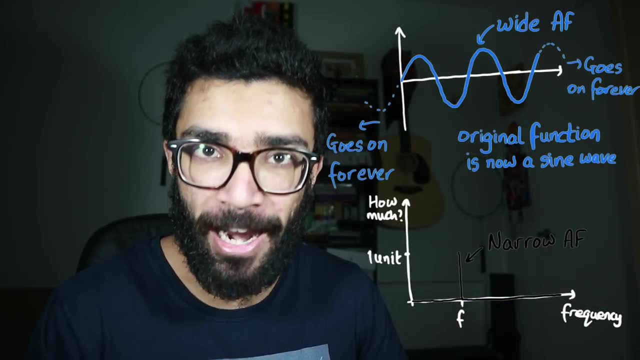 wave- the frequency of the original sine wave in this case, and it has no other sine wave frequency components. So our original function, a sine wave infinitely wide, has a Fourier transform that's infinitely narrow, It's peaked at one frequency and it has a value of zero at every other frequency. 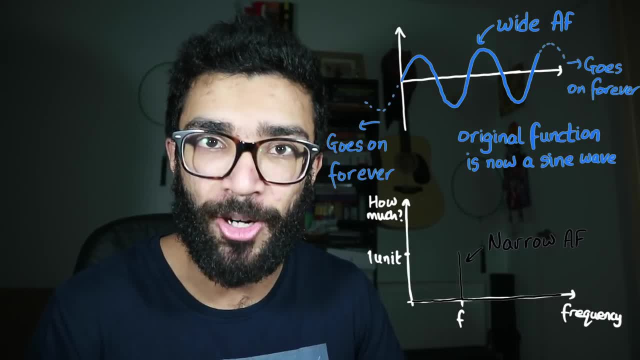 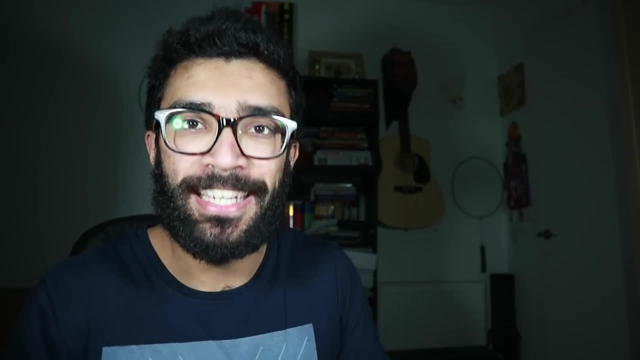 so it's infinitely narrow. So a wide original function results in a narrow Fourier transform, And this is true the other way around as well. by the way, If you have a narrow original function, you get a wide Fourier transform. Let's bring this back and link it to Heisenberg's uncertainty principle. To do this, we first need 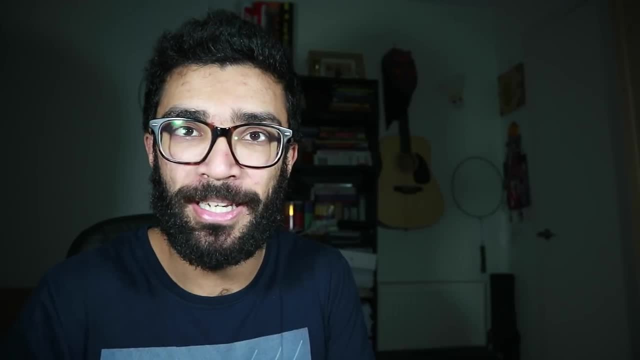 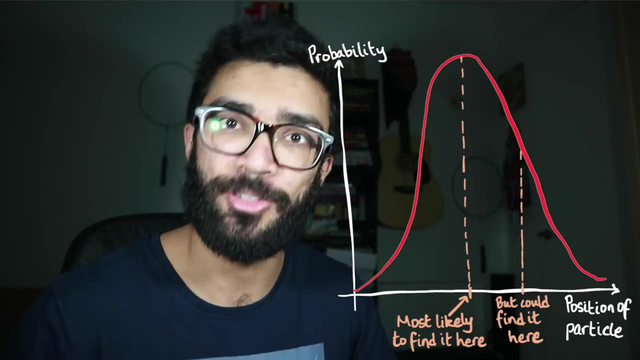 to remember what we said earlier about a particle's position and momentum being described by a probability distribution. In other words, we have a certain probability of a particle's position being in a range of values, and the same is true for its momentum. Now these probability. 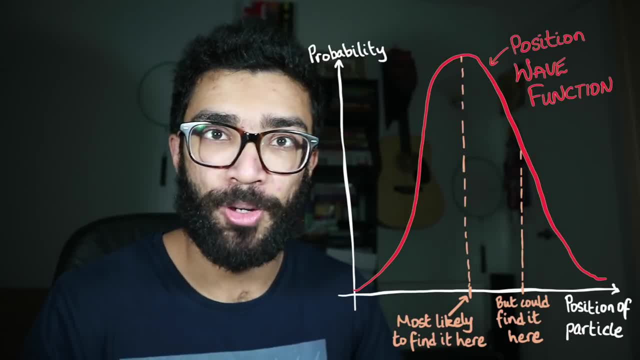 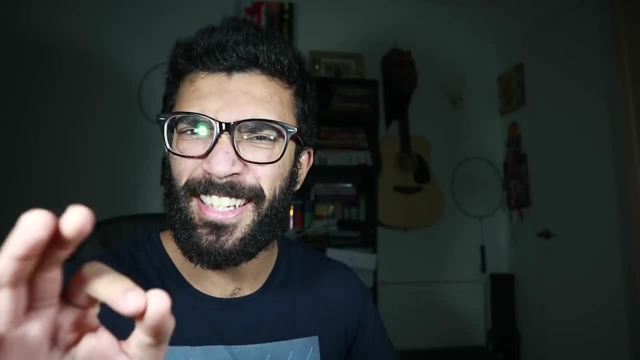 distributions are known as wave functions. So the wave function for a particle's position basically tells us the probability with which we'll find the particle in a certain position, and the same is true for the momentum. Now here's the clincher: The wave function for a particle's 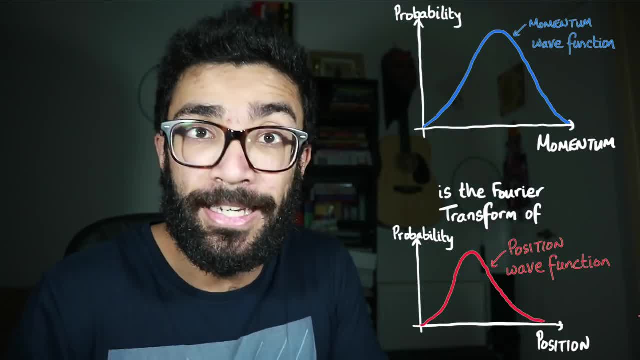 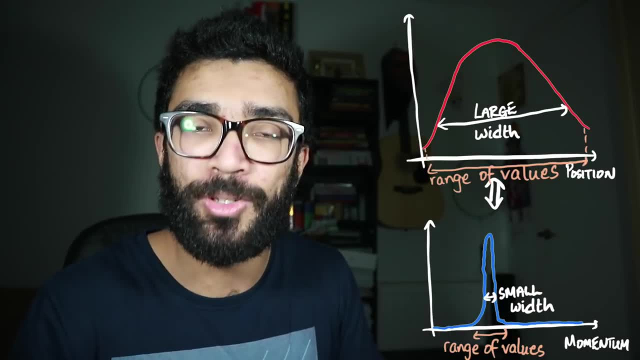 position is the Fourier transform of the wave function for the particle's position. In other words, if the wave function for a particle's position is wide, so we have less information about it because it could be in a large range of values, then the wave function of the particle's 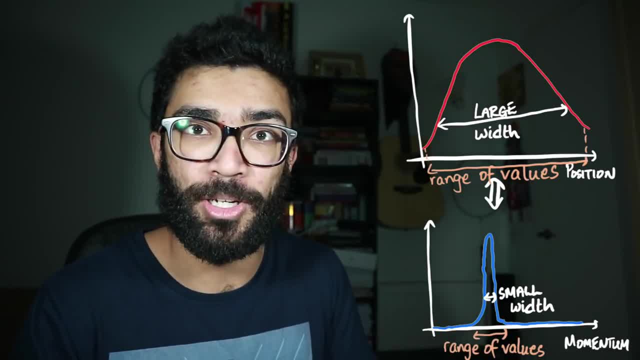 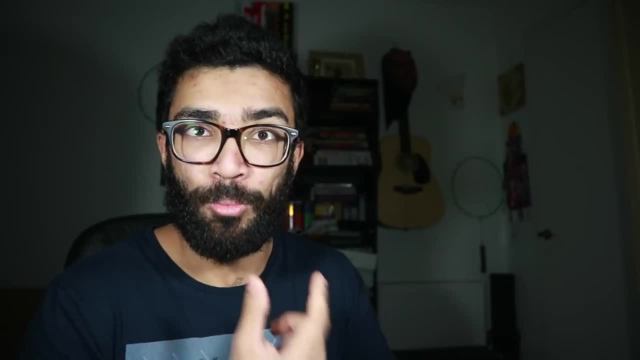 momentum is very narrow. In other words, we know a lot more about it. We're a lot more certain about the momentum because it could be in a very small range of values. And again, the opposite applies as well: Narrow position wave function. wide momentum wave function. The more we know about.